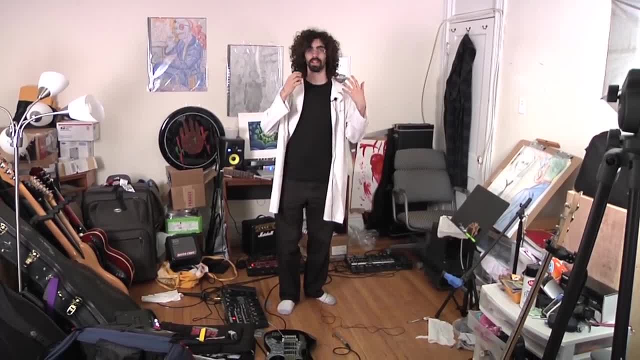 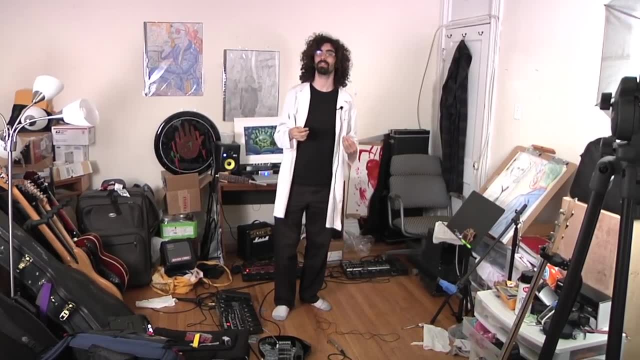 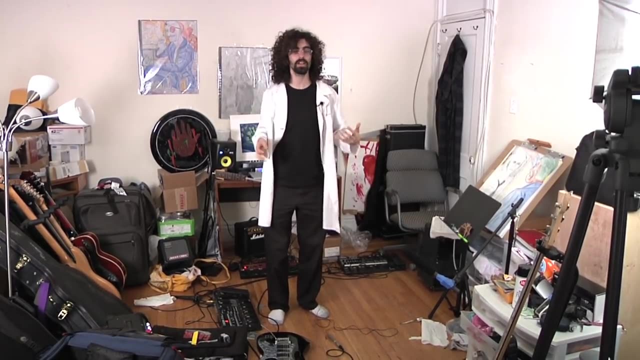 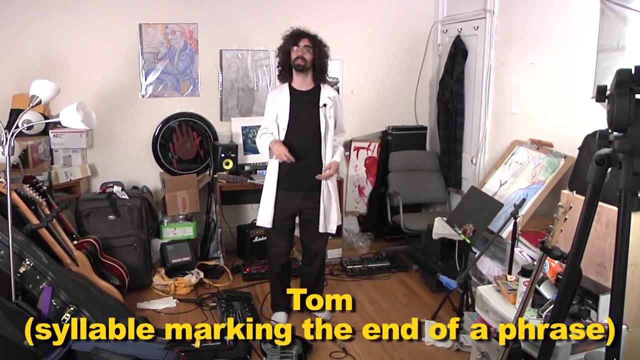 About music similar to the idea of Do Re Mi Fa Sol La Ti Do, which is just tonal solfege or whatever rhythmic solfege is taught specifically to teach rhythms. So instead of Do Re Mi Fa Sol La Ti Do, you have Ta Ta Ka Ta Ki. Ta Ta Ka Di Mi Ta Ri Ni Na Tam Ta Ki Ta Ta Ki. Ta Ta Ki Di Mi Ta Ki Ju Na Dum. 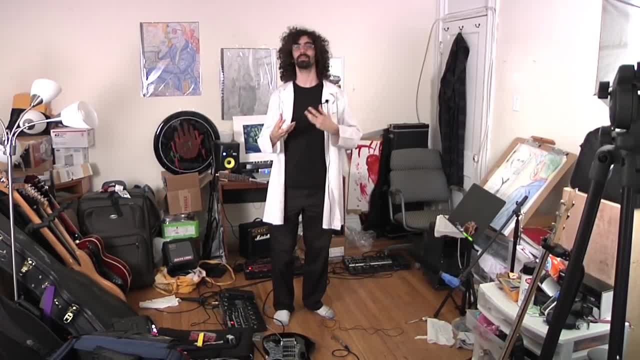 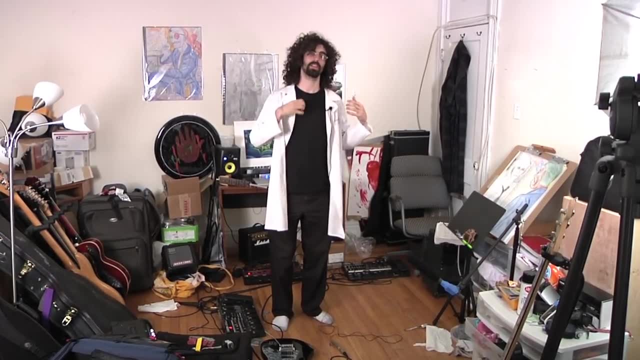 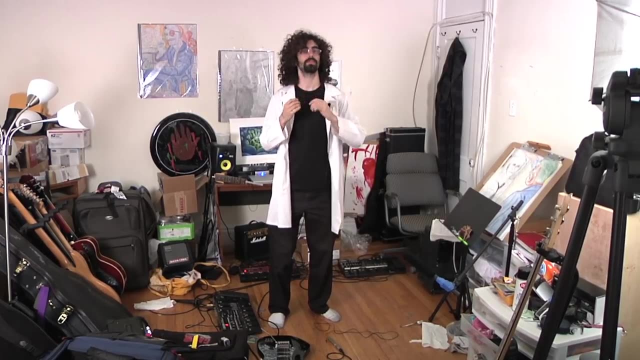 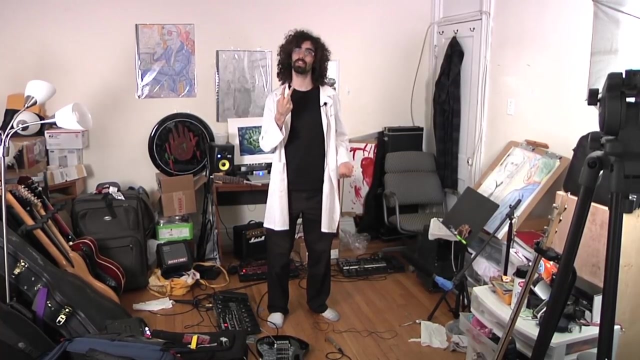 You know different kinds of rhythmic syllables that help you get muscle memory and all kinds of brain connections with how the rhythms feel and how they sound and how your body expresses them. So for groupings of one beat you typically would go Ta Ta, Ta, Ta. For groupings of two beats it'd be Ta Ka. 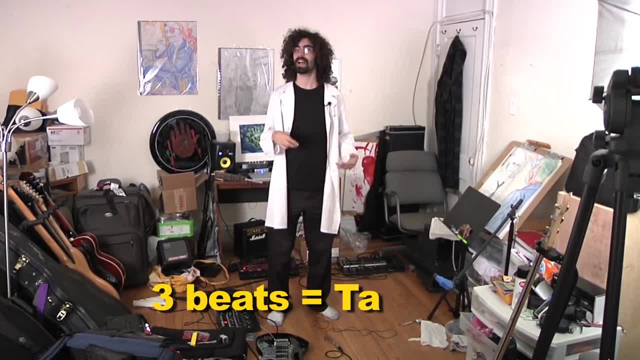 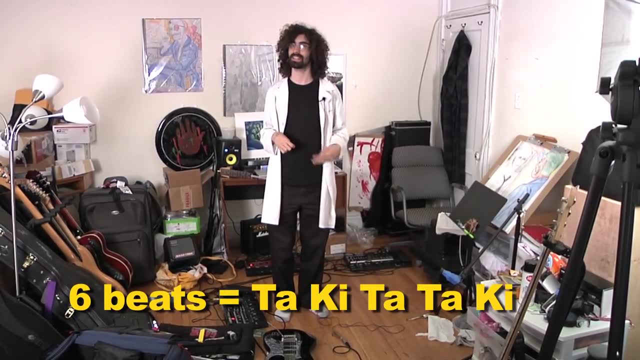 Ta Ka. Groupings of three would be Ta Ki Ta. Four, Ta Ka Di Mi, Five, Ta Di Ni Na. Tom Six is Ta Ki Ta, Ta Ki Ta. Seven is Ta Ka Di Mi, Ta Ki Ta. And eight would be Ta Ka Di Mi, Ta Ka Ju Nu. 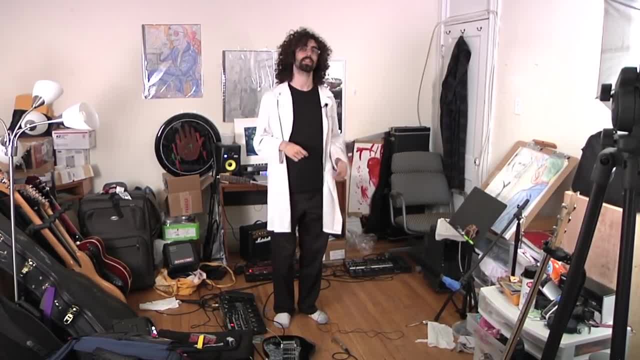 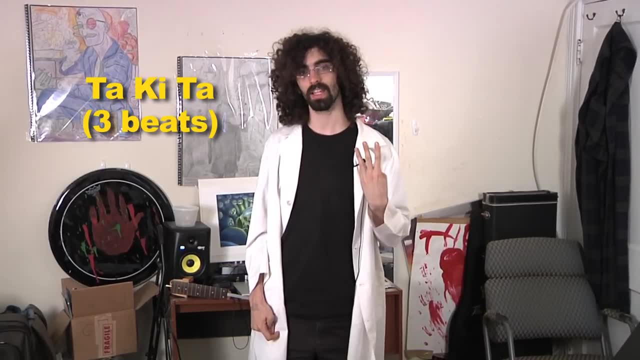 So you can use these groupings in two different ways. For example, you could have a phrase like: let's say Ta Ki Ta for three and Ta Ri Ni Na Tom for five, And together they'd go Ta Ki Ta, Ta Ri Ni Na Tom. 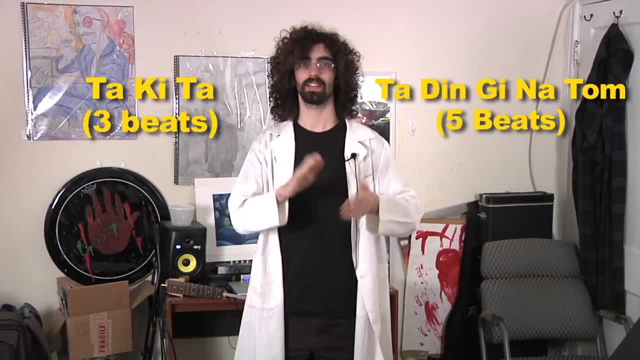 Ta Ki Ta Ta Ri Ni Na Tom. So if the quarter note is one-ee and a two-ee and a three-ee and a four-ee and a Ta Ki Ta Ta Ri Ni Na Tom. 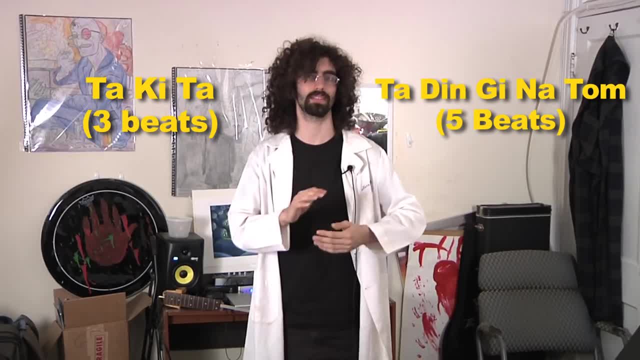 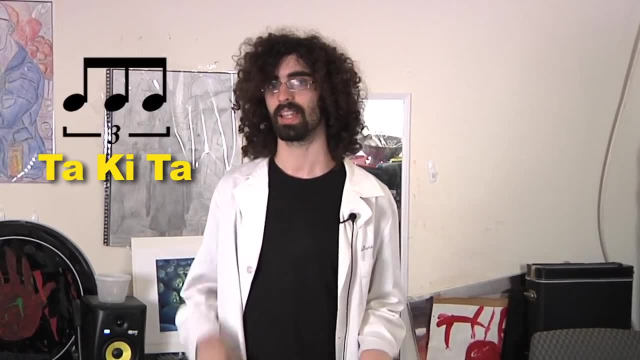 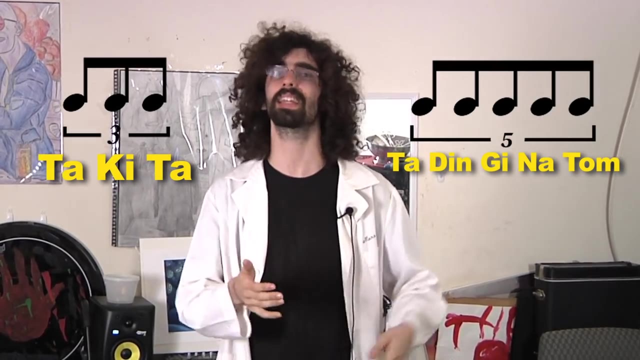 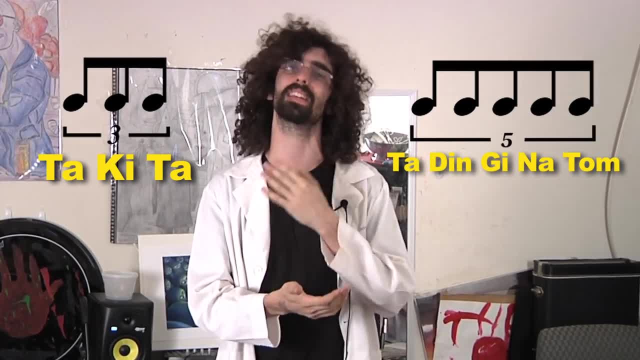 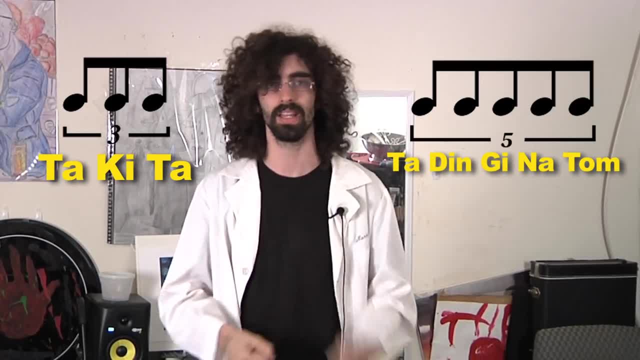 Ta Ki Ta Ta Ri Ni Na Tom Ta Ki Ta Ta Ri Ni Na Tom. Ta Ki Ta Ri Ni Na Tom, In which case the three is a triplet and the five is a quintuplet. 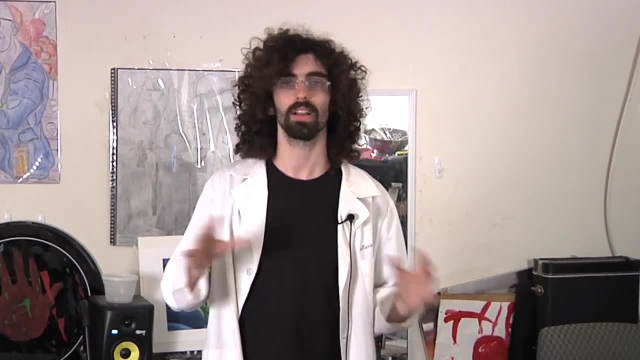 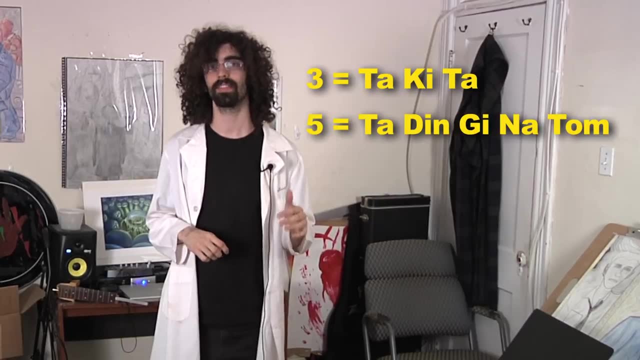 So using these two approaches we can make all kinds of cool rhythms. Let's take a grouping, We'll keep straight sixteenth notes. Let's do three, five and then seven. Three will be Ta Ki Ta, Five will be Ta Ri Ni Na Tom. 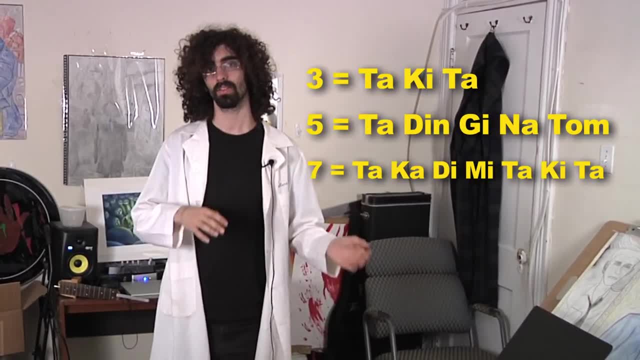 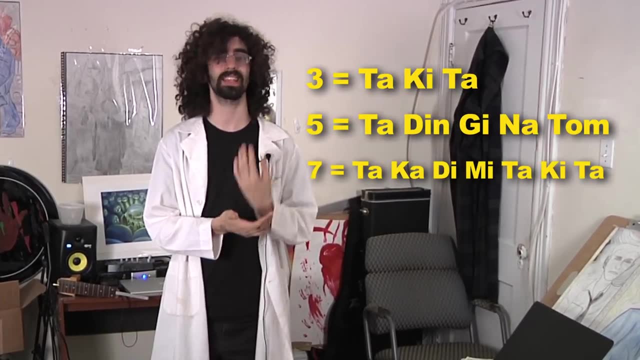 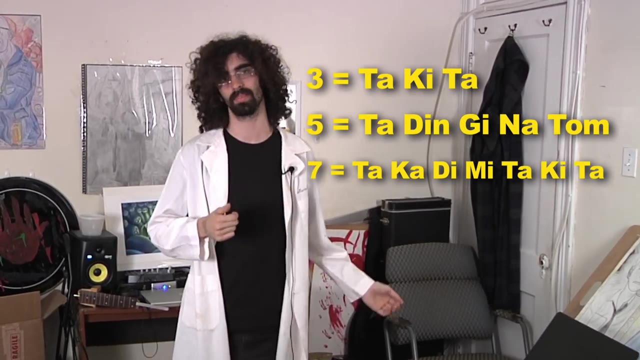 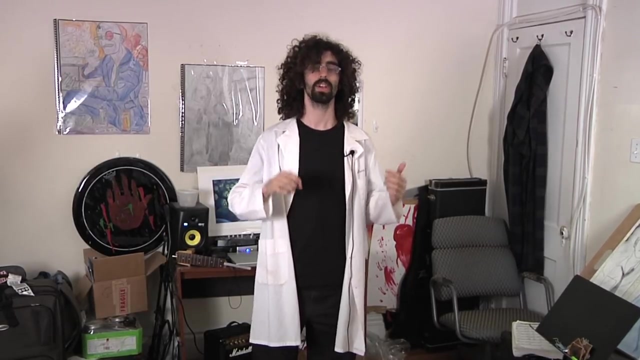 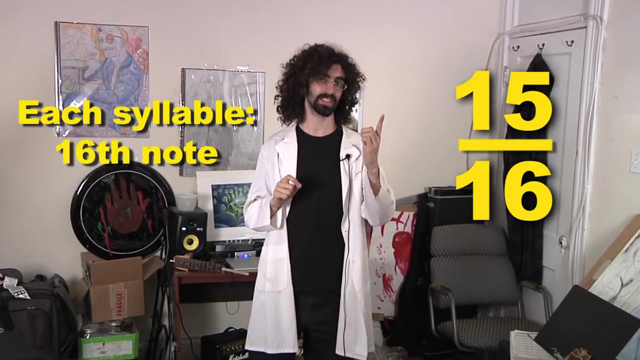 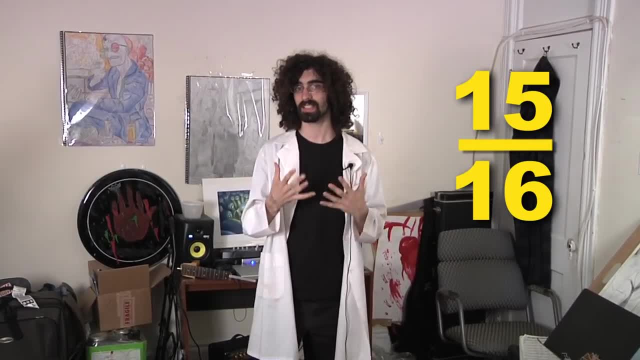 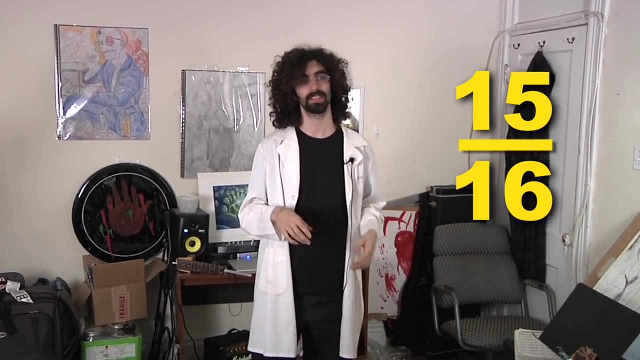 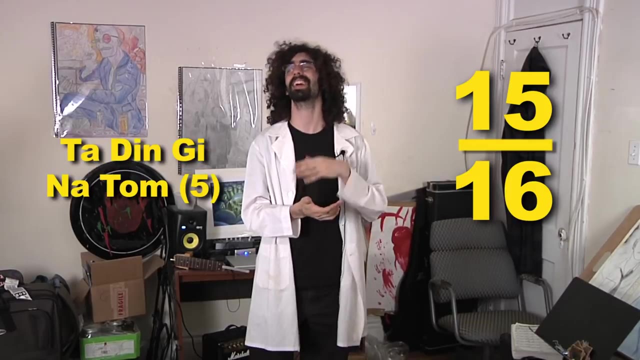 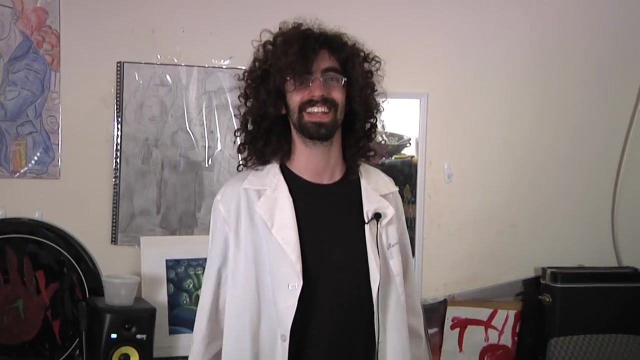 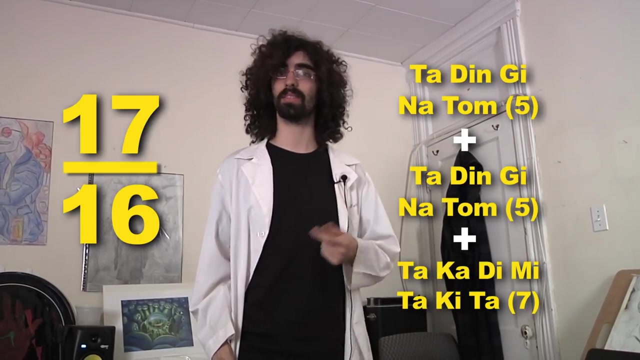 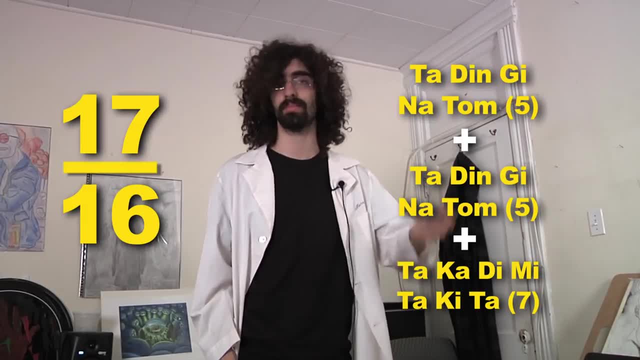 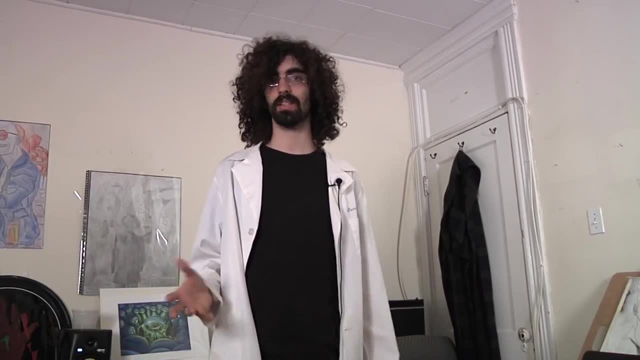 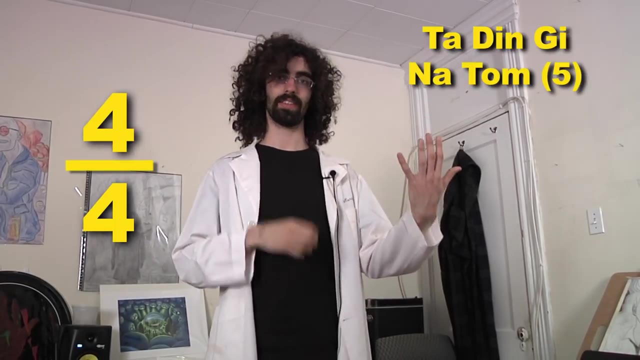 so those were measures of 17. now let's take an easier time signature like for four and make a cool way of doing four-four. one of my favorites is five, three, three, five, five and three equals 8 16ths. then three and five equals 8 more. 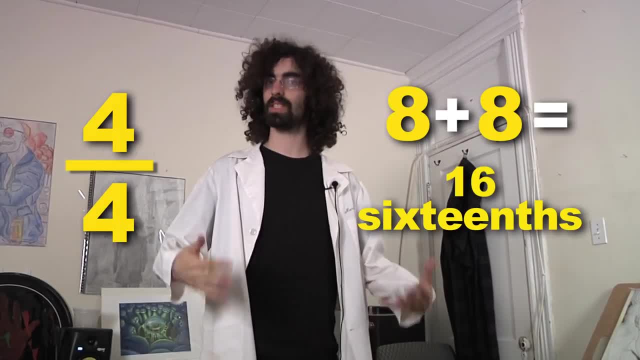 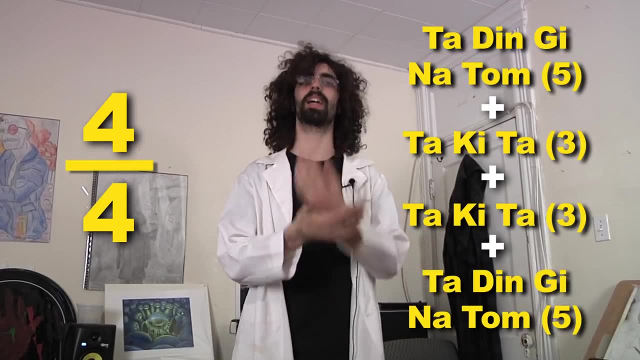 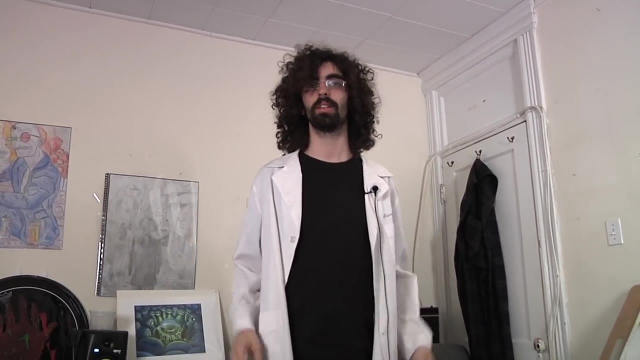 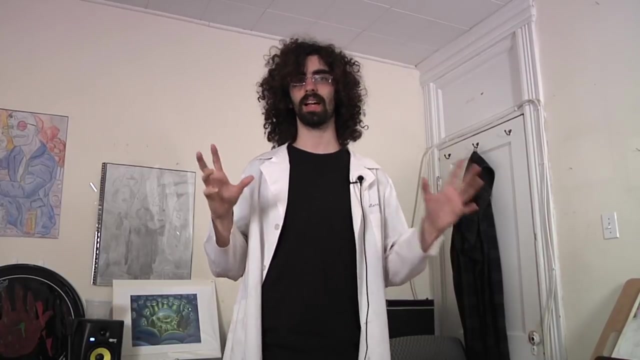 sixteenths. combine that together, you have 16 sixteenths, which is equal to a, a measure of four-four. So that's a really cool way to divide something simple like four-four. Four-four, you'll find, is like an incredible time signature, even though it's common. there's. 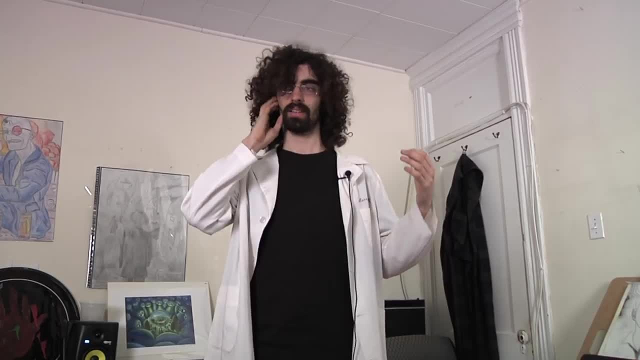 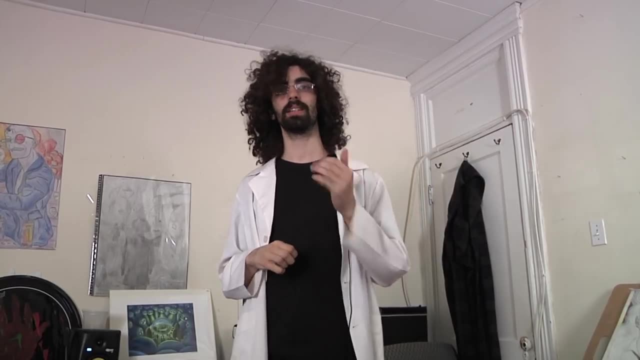 so much you can do with it. You just take a number like two numbers that add up to eight or two numbers that add up to sixteen, you apply the syllables to them and then you can use those to set the subdivisions and the accents that you're going to use. 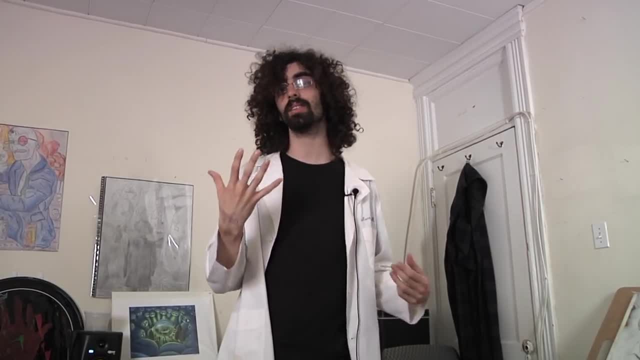 Now the other way we did it, where ta-ki-ta-i was a triplet and then ta-di-ngi-na-to-m was a quintuplet, or ta-ka-di-mi could be sixteenths. you know, when we change it that way now. 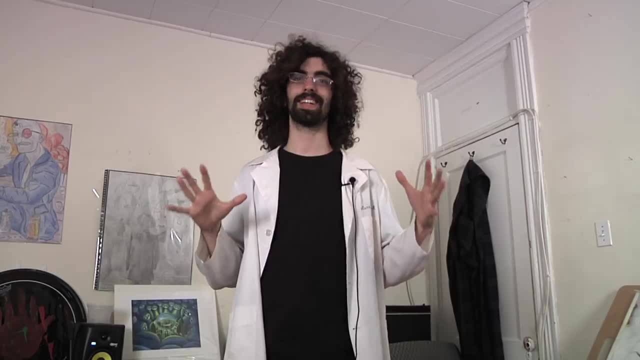 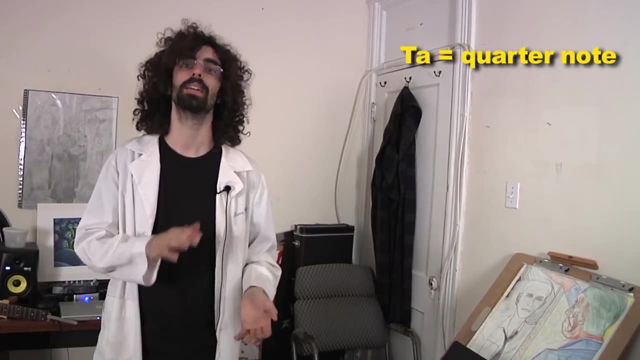 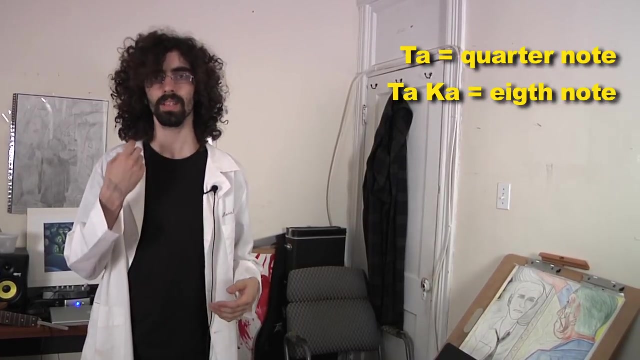 we can get into some really cool like accelerating and slowing down time, manipulating kind of ideas. So tau will be a quarter note. Ta, ta, ta, ta, ta-ka will be an eighth note. ta-ka, ta-ka, ta-ka, ta-ka, ta-ki-ta will be. 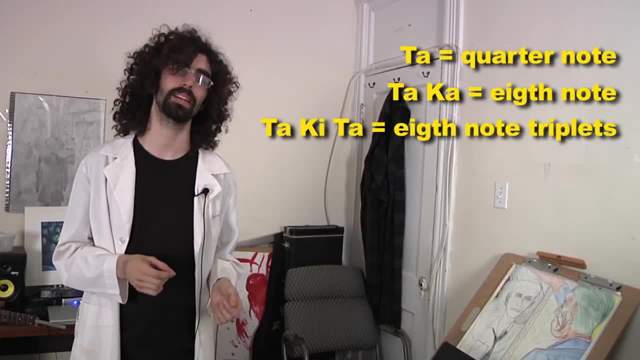 eighth note triplets: ta-ki-ta, ta-ki-ta, ta-ki-ta, ta-ki-ta, ta-ka-di-mi will be sixteenth notes: ta-ka-di-mi, ta-ka-di-mi, ta-ka-di-mi, ta-ka-di-mi, ta-ka-di-mi, ta-di-ngi-na-to-m. 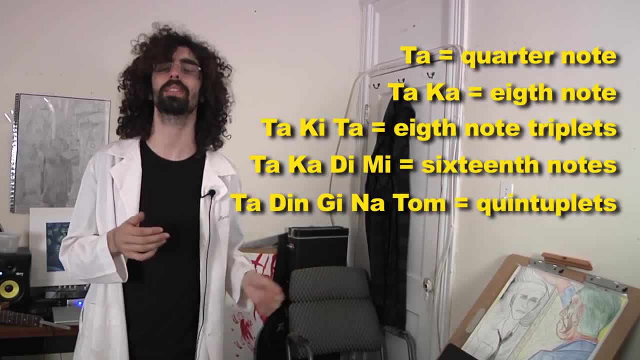 will be quintuplets: ta-ni-ngi-na-to-m, ta-ni-ngi-na-to-m, ta-ni-ngi-na-to-m, ta-ni-ngi-na-to-m, ta-ki-ta- ta-ki-ta will be sixteenth note: triplets: ta-ki-ta- ta-ki-ta, ta-ki-ta, ta-ki-ta. 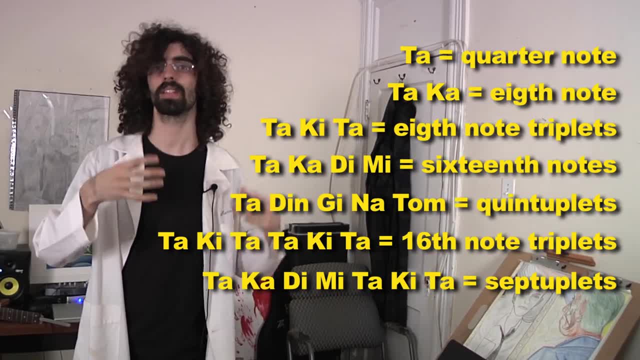 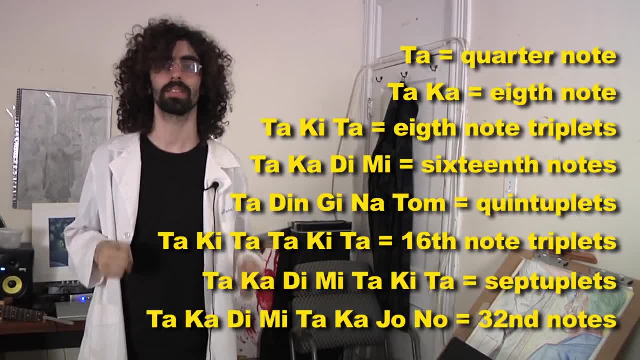 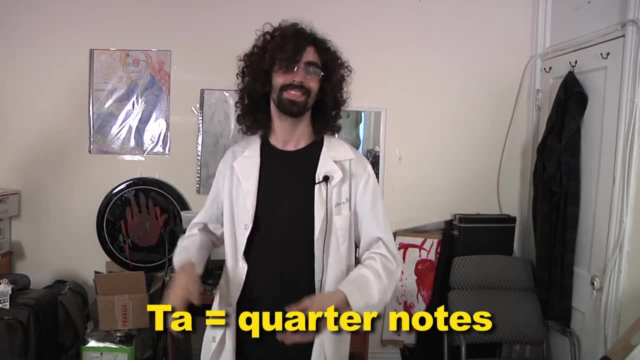